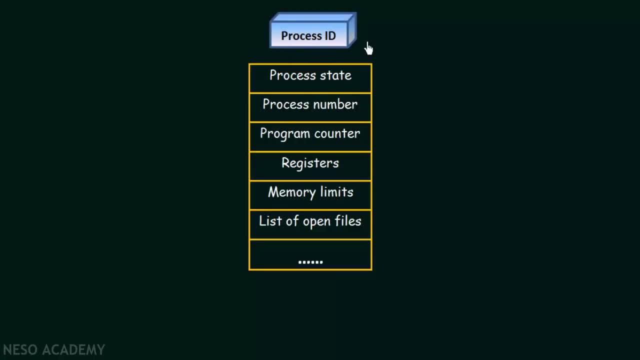 So the first thing that we have is a process ID. So process ID or process number, as it is given in this example, it shows the unique number or unique ID of a particular process. So every process has to be represented by a. 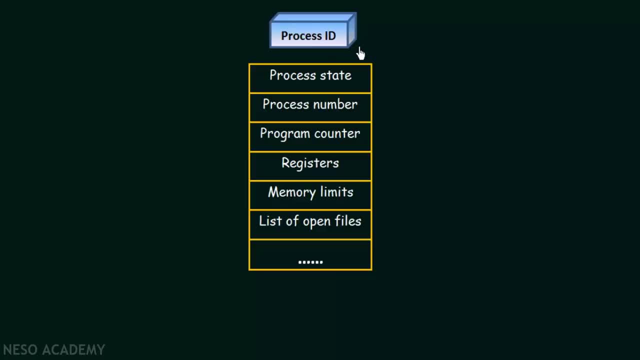 process ID, which will identify that process. So this process ID is the unique number or identification that identifies a particular process, and this is one of the things that is present in a process control block, which is used to represent a particular process. Now, the next one that we have is process state. 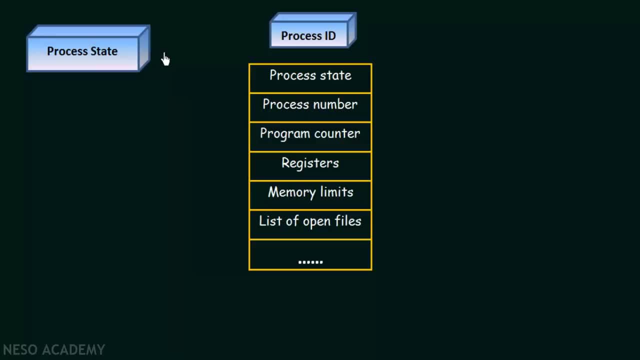 So what is process state? Process state tells us the particular state in which a process is at that particular moment. Now, in the previous lectures we studied about process state and we saw that a process can be in different states, like the new state, running state, waiting state, terminated state and so on. 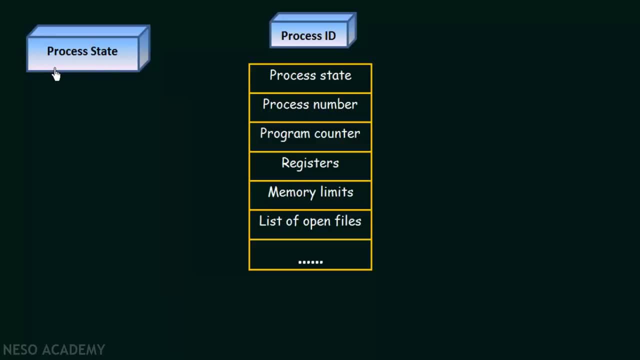 So this process state will tell in which of those states is the process in at that particular moment. So this is also another thing that is there in the process control block, which will represent a particular process. So the next one that we have is a program counter. 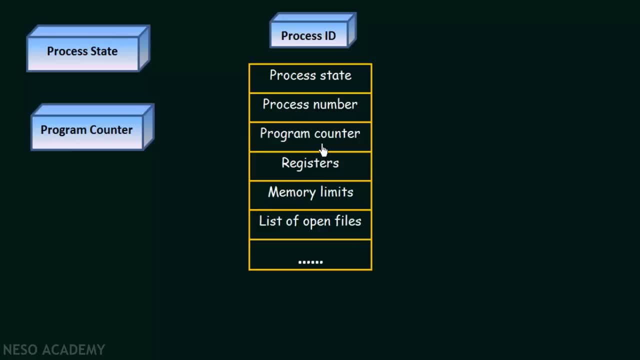 So the program counter. it indicates the address of the next instruction that has to be executed for that particular process. Now let me explain what this means. Now we already studied that a process is a program in execution. When a program is in execution, 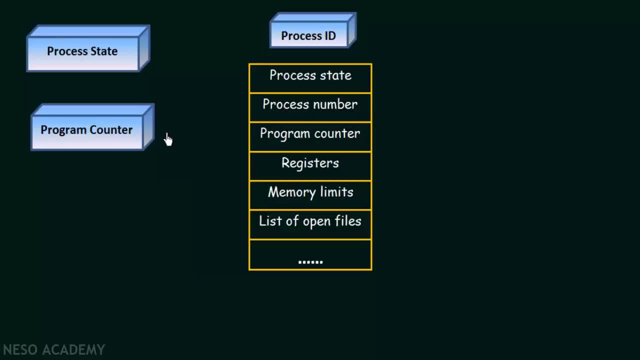 at that moment. we call it a process. So when a process is being executed, the lines of instructions or the lines of codes are executed line by line. Now, when it is being executed, this program counter tells us the address of the next line of instruction. 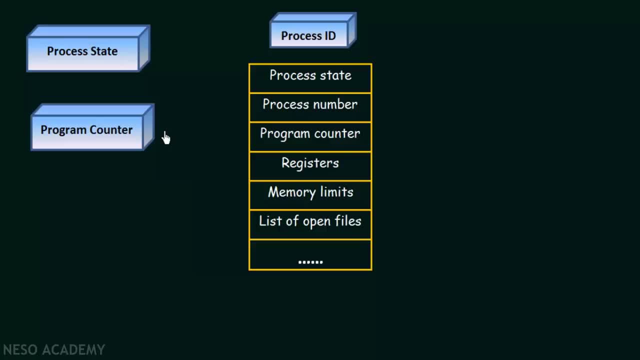 that has to be executed. So we have lines of instructions that are being executed and at a particular moment, what is the address of the next line that has to be executed? That is given by the program counter. So the program counter indicates the address of the 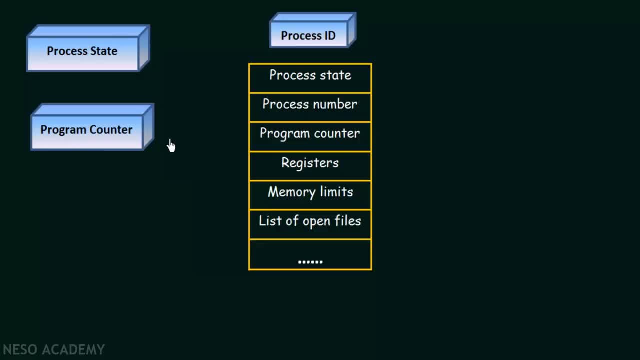 next line of instruction that has to be executed for a particular process. Alright, so the next one that we have is CPU registers. So CPU registers tells us the registers that are being used by a particular process. So there are different kind of registers, like the index registers. 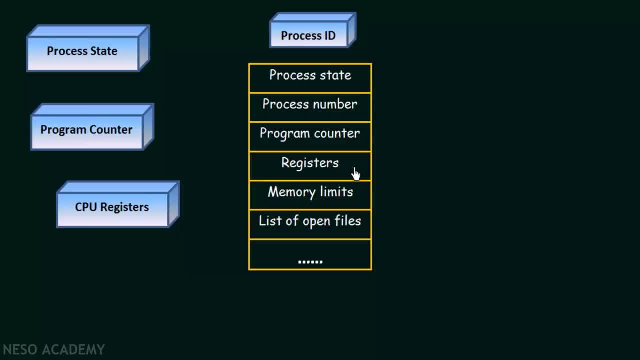 stack pointers, general purpose registers and so on. So these CPU registers will tell us the particular registers that are being used by a particular process. So this is also another thing that we have in the process control block. So the next one that we have is CPU scheduling information. 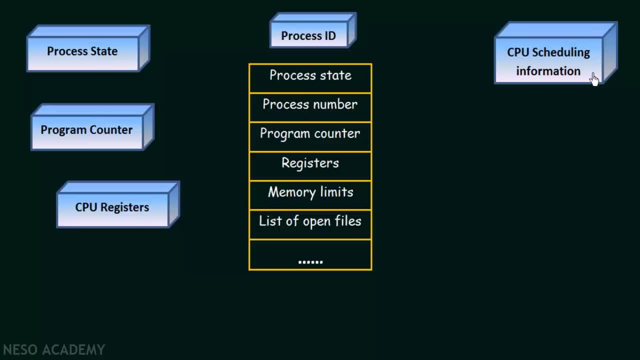 So this CPU scheduling information has the priority of the processes. It has the pointer to the process control block, It has the pointer to the scheduling queue and also other scheduling parameters. Now, scheduling is a very important topic as far as operating system is concerned. 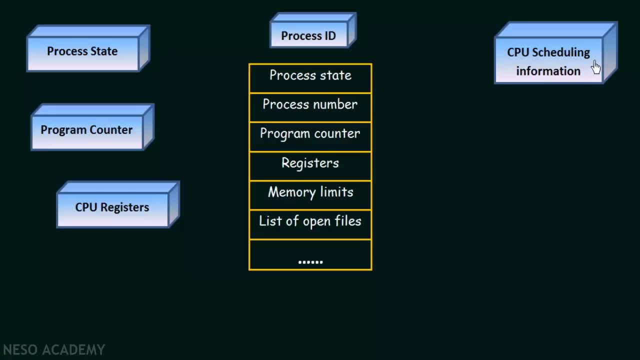 and there will be a whole topic regarding it, which we will be discussing later, But for now, let me give you a brief idea of what scheduling is. So we know that there are many processes that are waiting to be executed. It's not only one process, but there are many processes. 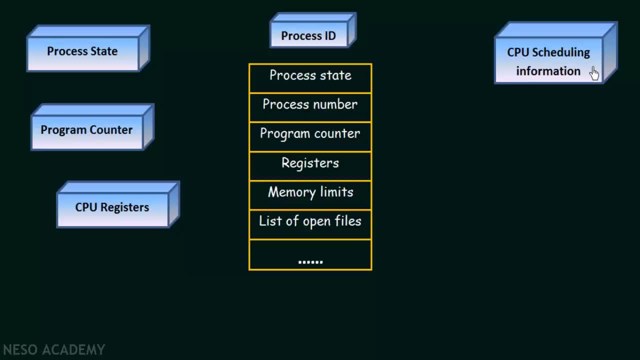 that are waiting to be executed. So scheduling determines which process has to be executed first, or it determines the order in which the processes has to be executed. So there may be processes with higher priority than other processes, So they may have to be executed first. 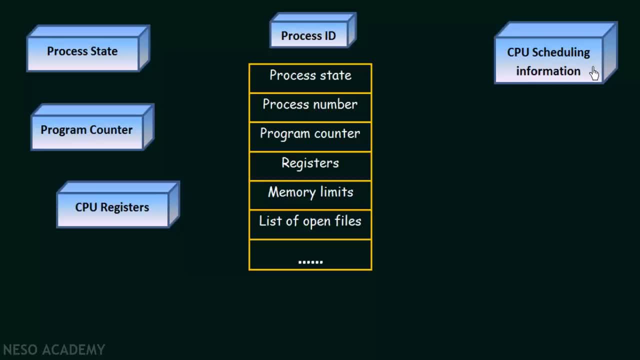 And also when processes are all waiting in a queue, it has to be determined how much time has to be allotted to a particular process, And all those kind of things are determined by the scheduling algorithms. So that is what we mean by scheduling. 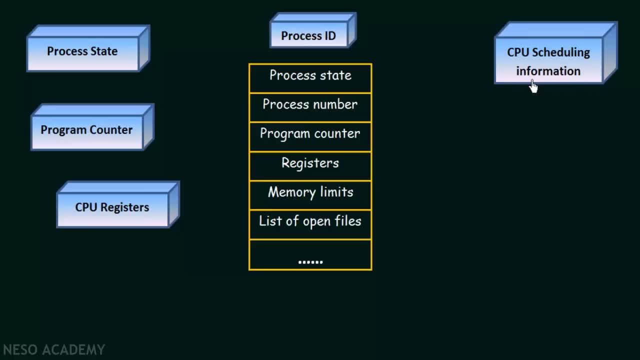 And so the CPU scheduling information is also stored in the process control block. It is not shown in this example over here, but this is also another thing that we have in the process control block Now. next we have the memory management information. So the memory management information. 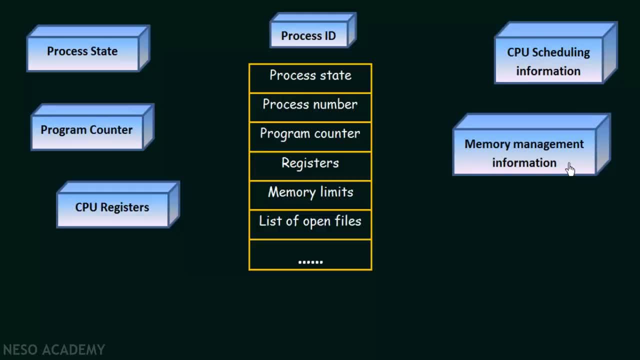 from the name itself. you must have understood. It represents the memory that is being used by a particular process. So different aspects of the memory, all those information regarding that will be stored in the memory management information And that is another thing that is stored in the process control block. 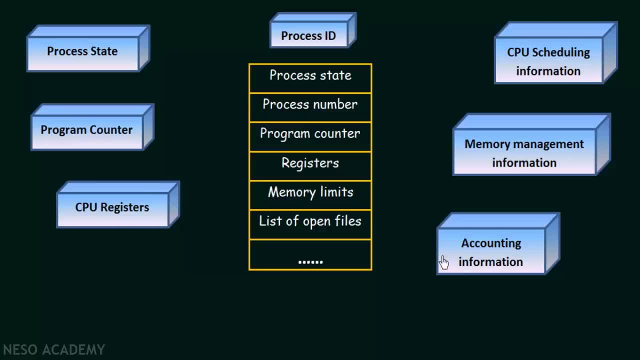 Now. next, we have accounting information. So this is also not shown in this example, but we have the accounting information. So accounting information keeps an account of certain things, like the resources that are being used by the particular process. So there are different resources that are used.